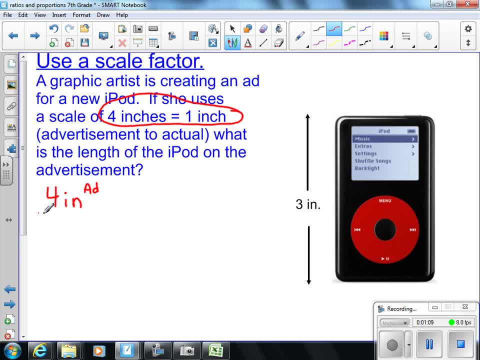 4 inches- this is in the ad, or the advertisement- compared to 1 inch and this is in the real world. This is like the actual. Okay, then over here. this is like the real thing. In reality, your iPod is going to be about how tall or how long. 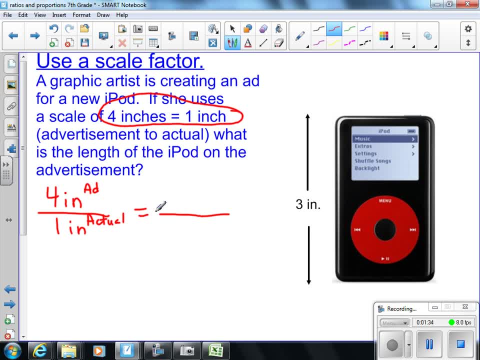 3 inches. So will that go on the top or on the bottom? On the bottom, because it's in real life or the actual thing. We're going to put 3 inches, So we do not know how many inches the ad is going to be, and that's what we're going to find out. 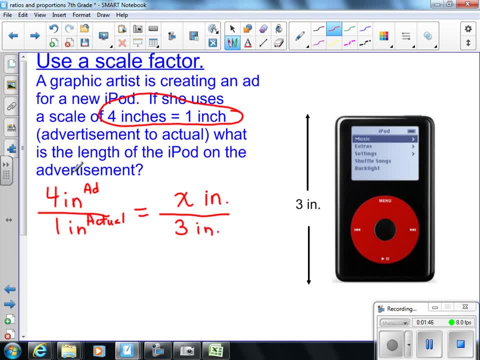 Because that's what it says. The question is: what is the length of the iPod on the advertisement? Okay, so now we're going to use what to solve Cross products. Okay, so now we're going to use what to solve Cross products. 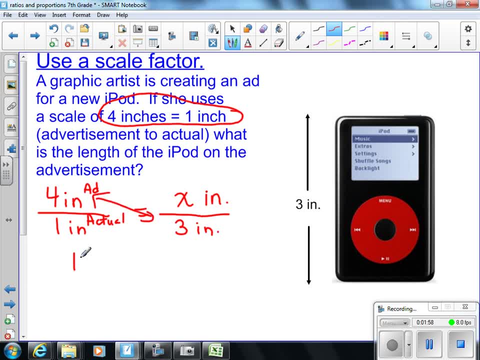 Now let's start with: 4 times 3 equals 12, and then 1 times x is 1x. Okay, write that down. Now what am I going to do to both sides to solve Divide by 1.. Divide by 1,: good. 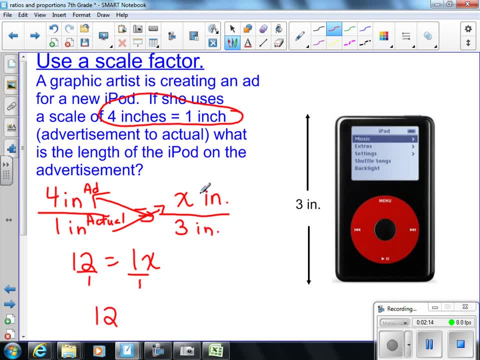 So I get: 12 is equal to x. 12. what? What will my label be? 12 inches equals x, Or 12 inches will be how tall the ad will be? Okay, are there any questions? Alright, so basically, if you're given a scale, you can use that scale to help you solve problems. 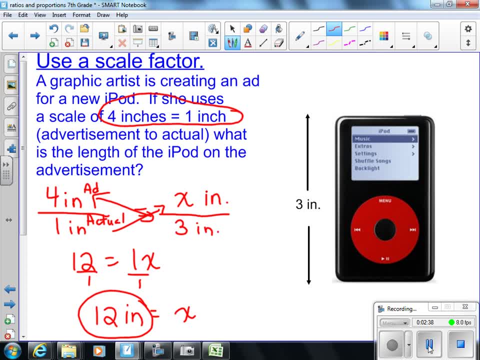 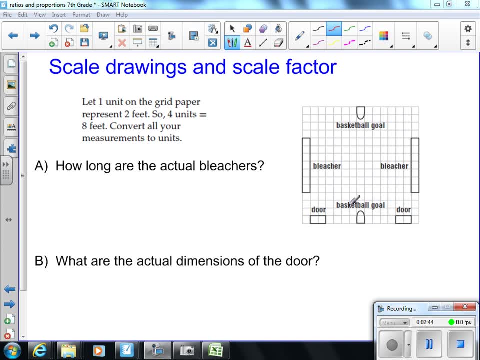 Okay, and you set up a proportion in order to do so. Alright, so let's take a look at another example. This time, they give us a picture. Okay, this is not the real thing. Okay, this is the picture. They're telling us, though, that one unit on this grid is going to represent actually 2 feet in reality. 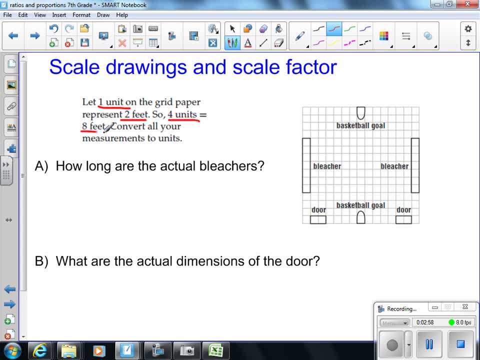 Or they tell us that 4 units on the grid will be equal to 8 feet. in reality, Is that pretty much the same thing: If I have 1 unit, that's going to be 2.. If I have 4, that's going to be 8.. 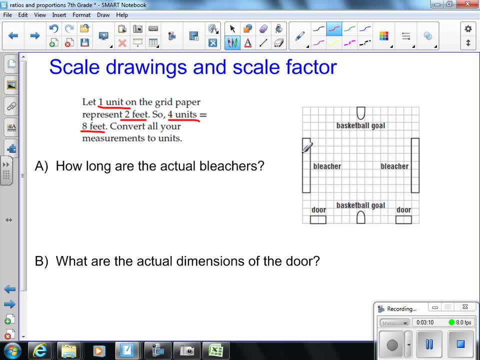 Does that make sense? Now we're going to convert all of our measurements to units here and we're going to answer these questions: How long are the actual bleachers? Now we're just going to look at one set: How long are these bleachers? 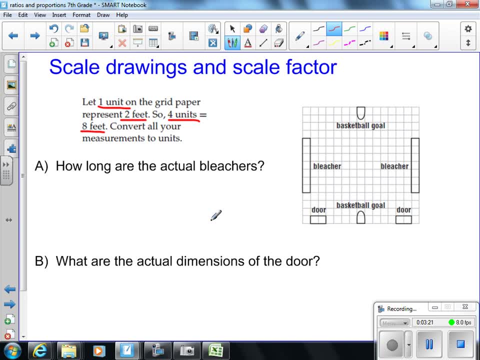 Well, again, find your key or your rate or ratio that they give you. What is the comparison that they give you? I could either use 4 units to 8 feet, or somebody else said you could use 1 unit to 2 feet. 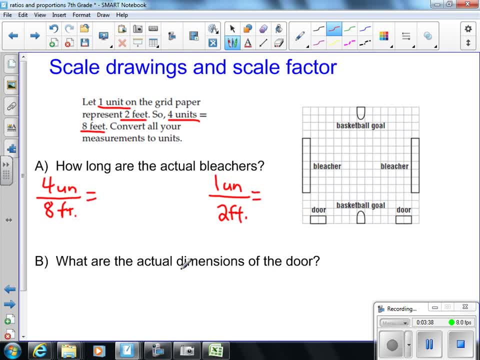 So I'm going to work it both ways. So I need to have units on top feet on the bottom, Units on top feet on the bottom, Okay, so how many units are my bleachers here? Okay, you count 7.. 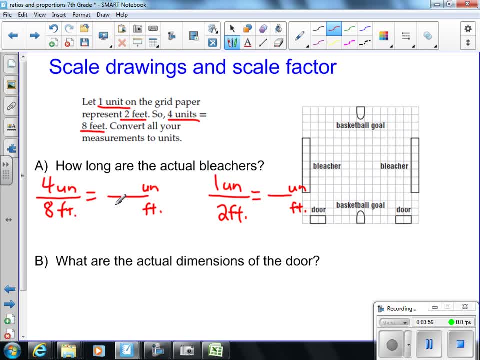 1,, 2,, 3,, 4,, 5,, 6, 7.. Okay so, will it go on top or bottom, Top, Top or bottom over here, Top. Okay, so then this is your unknown. 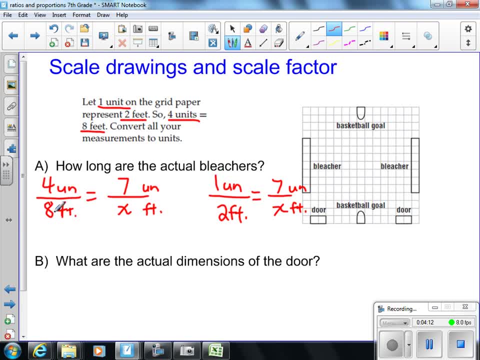 Alright, let's work this one, the first one. We'll go ahead and do it first. 8 times 7 is 56 equals 4x. So what do I need to do? to both sides, Divide by 4.. Everybody got that. 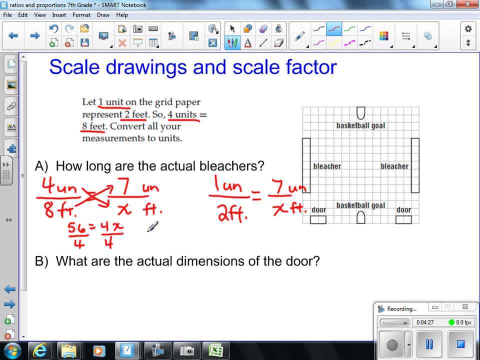 What's 56 divided by 4?? Got it 14, what? Look at your label so you can tell by where your variable is 14 feet. Let's see if we get the same thing if we do it this way. What's 2 times 7?? 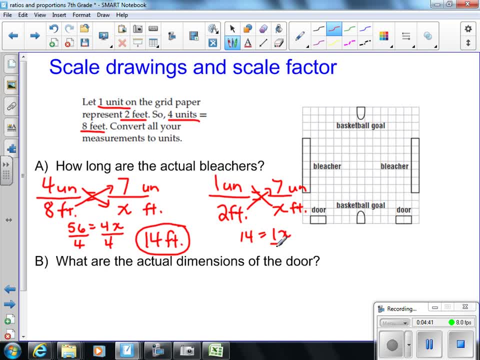 Equals 1 times x divided by 1.. And you get 14 feet again. So did it matter which one of the ratios you used? Not if they're representing the same thing, It doesn't matter. Okay. so how long are the actual bleachers? 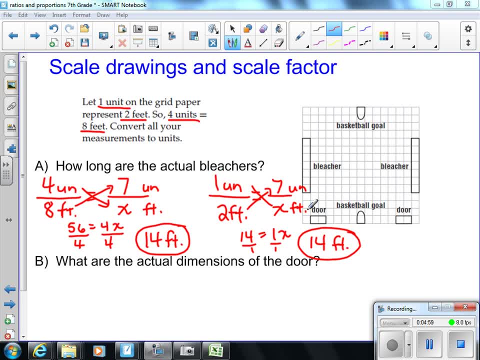 I'm thinking they're asking me: just one set of bleachers is how long? Okay, yes, That would be a good thing. They're 14 feet long each. That might be a good thing to add, And if you have that on a test or a quiz, I think that's something that you might ask. 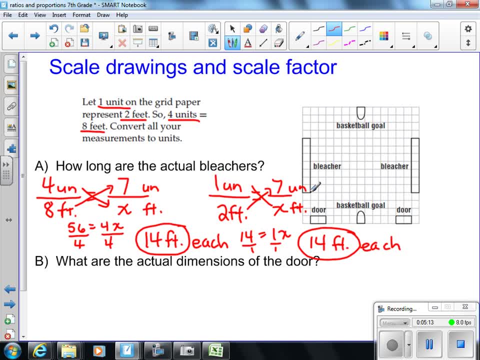 Clarify and say: is this just referring to one set of bleachers? How long are the sets of bleachers, Or do they want both of them combined? All right, now let's look at the actual dimensions of the door. Let's start with the 1 to 2 ratio this time. 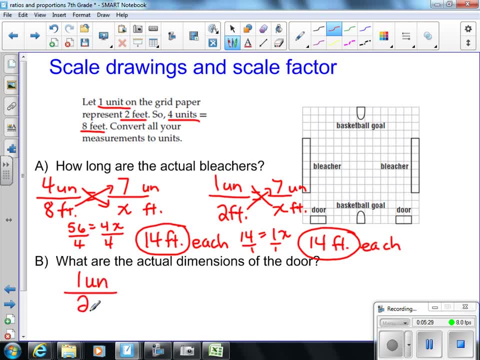 1 unit to 2 feet will be equivalent to units over feet. Okay, find the doors. What are the dimensions of the door? Okay, 2 units. So we have 2 units here, x down here. Use cross products. 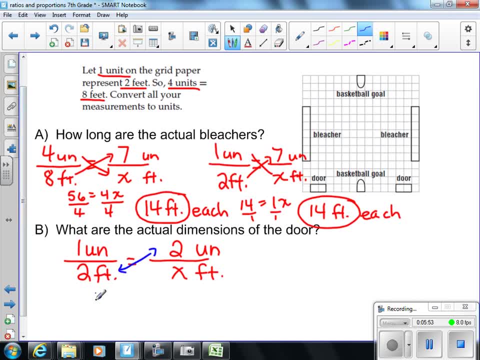 Okay, 2 times 2 is 4.. 1 times x, 1x Divide by 1 and you get 4 feet is the width of the door If we had each one. It just wants to know what's the actual dimension of a door, of the door. 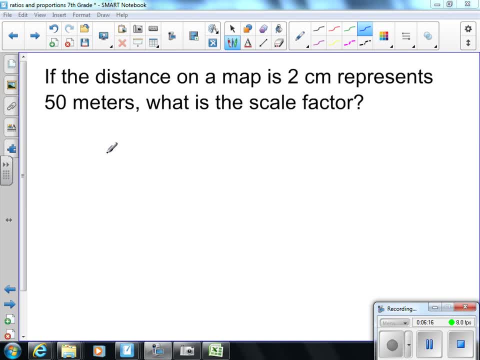 Okay, now we've been working on scales and using the scale to help you establish your new links, Let's take a look at what is a scale factor. A scale factor is something that you take times an amount in order to get your new amount. 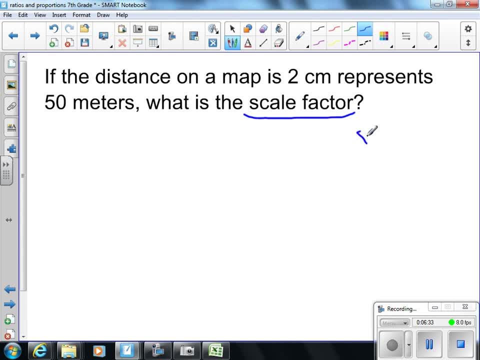 Like say, for instance, that I have a little cricket sitting here on the floor. Okay, here's a little cricket, You know he's got his little head. No, there's his little legs or something. My little cricket's sitting here. 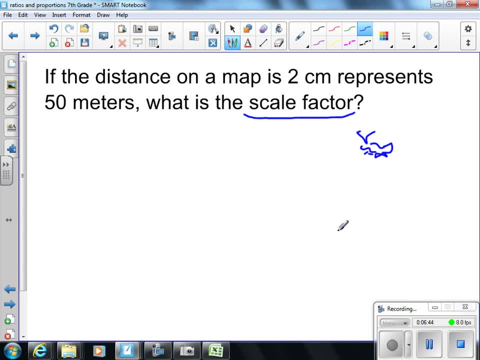 And I'm going to draw a picture of him, But I'm going to fill up an 8 by 11 sheet paper. Would I be making an enlargement or a reduction? I'd be making an enlargement. I'd be making an enlargement. 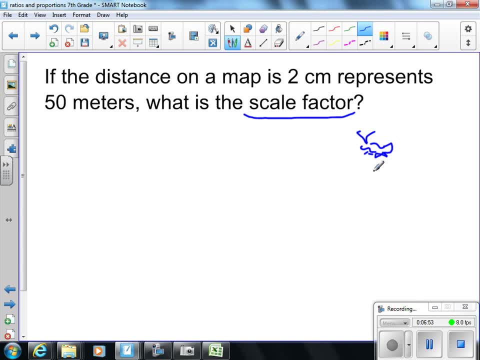 So the number or the scale factor I would take my measurement on my real cricket by would be a whole number or a big number Like it'd be 10 times, maybe as big as what it was originally. But let's say, for instance, I have a real car sitting out here in the parking lot. 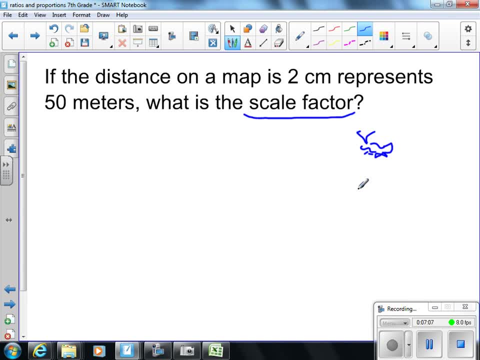 And I'm wanting to make a picture of it on my 8 by 11 sheet of paper. I would have a reduction, So I would be taking everything times a fraction, Like it might be 1- 16th. Do any of you collect those little toy tractors? 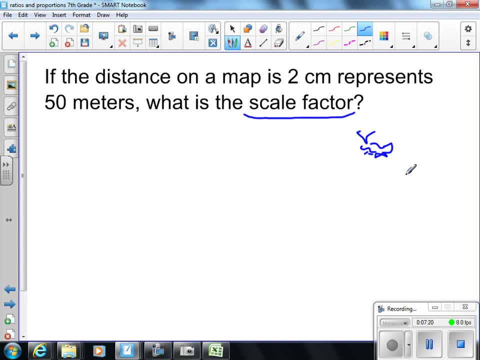 Or implements. They're sold by like 1 64ths of a size, Or 1 12th of a size, And that's why- Because that's the scale factor that those tractors or those little implements are made from. Okay, so let's take a look at this. 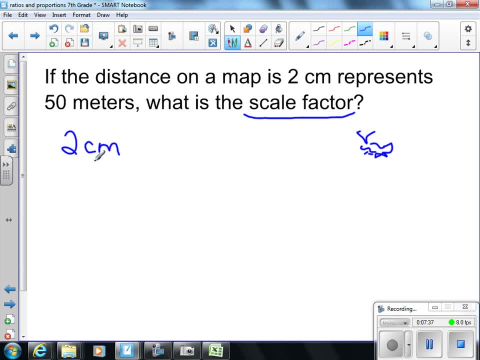 It says: if the distance on a map 2 centimeters represents 50 meters. We're wanting to find the scale factor, Not the scale, Because this could be considered a scale, Although usually you have 1 centimeter per meter. 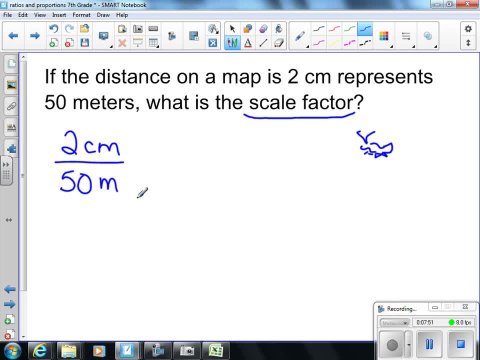 Or 25 meters would be the scale. Okay, The scale factor is what? would I take my dimension times to get my new one? So when I do that, I have to make sure that my units are the same. Okay, There can't be 1 centimeters or 1 meters. 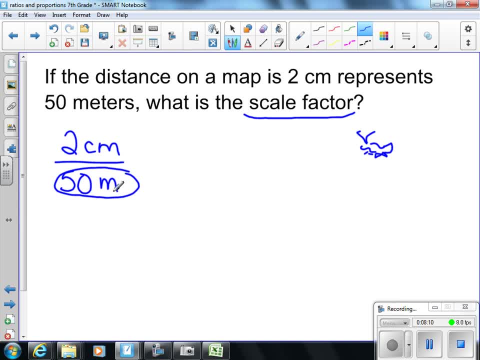 They both have to be. In this case, I'm going to make them both centimeters. Now you might ask: why didn't I make them both meters? I usually go with a smaller unit, Okay. So whichever one is smaller, Which I know, centimeters are smaller than meters. 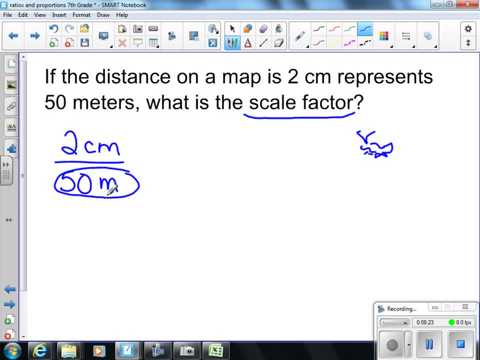 I'm going to make them both centimeters, Alright. So 50 meters is how many centimeters? 2 centimeters compared to 5,000 centimeters. Everybody remember King Henry died Monday drinking chocolate milk. Okay, So you do 2 hops. 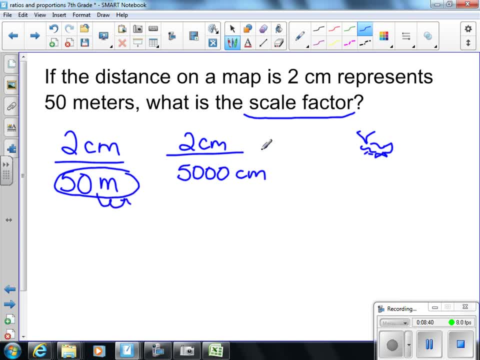 Right, And you get 5,000.. And then we try to simplify this. How can I simplify this? Divide them both by 2. And I get 1 centimeter to 2,500 centimeters. So what I would be doing is if I have a length on something, 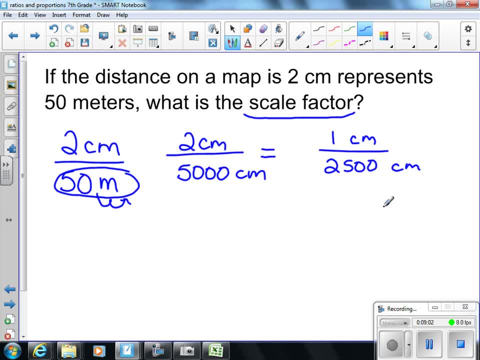 I would be taking it times 1 over 2,500. And I would be shrinking it. Okay, Because this is a fraction. I know that whatever I'm doing, I would be shrinking what I'm doing, Making it smaller. It would be a reduction. 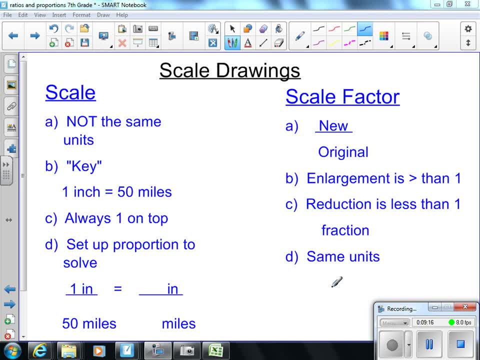 Okay, This is just what we've kind of gone over so far. Then we're going to do some more examples: Scale drawings. We've looked at 2 things. We've looked at scales, Which the scale is like the little key that you have on a map or a drawing. 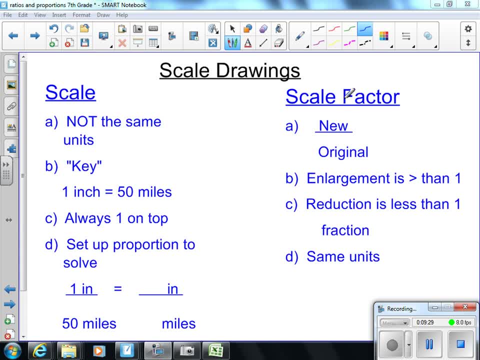 Where the scale factor is what is a fraction or a whole number, that you take your dimensions times to get your new numbers Now on the scale. On a scale, You don't necessarily have to have the same units, Okay, And often case you don't. 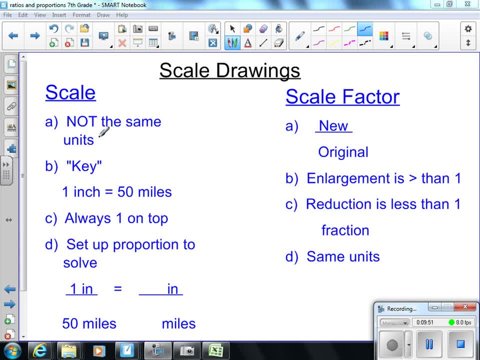 For instance, on a map, 1 inch is equal to 500 miles. Okay, So you don't have to compare. You're comparing inches to miles And they don't have to be the same. Usually it refers to a key In which you have like: 1 inch equals 50 miles. 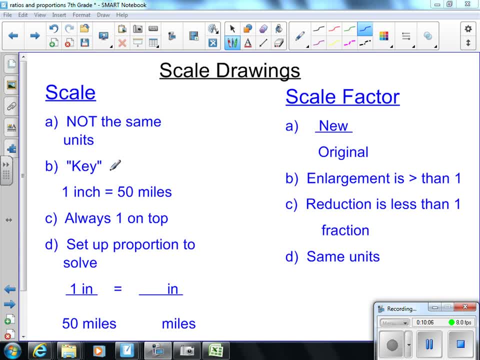 Sometimes we call the scale the same thing as a key, And always 1's on top. So, even if I started with, 2 centimeters is equal to 5 meters. You want it to be represented as: 1 centimeter is equal to how many meters? 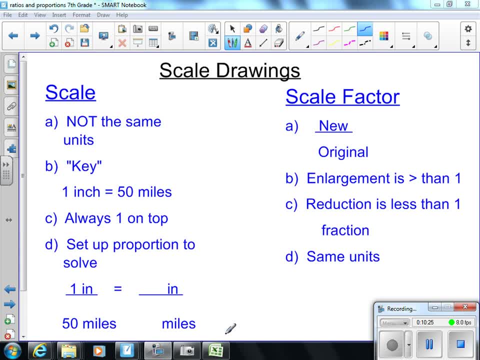 And sometimes, in the scale problems, you set up a proportion to solve. most often You'll set up a proportion to solve it. 1 inch represents 50 miles. Well then, how many inches on my drawing equals? tell me how many miles that'll be. 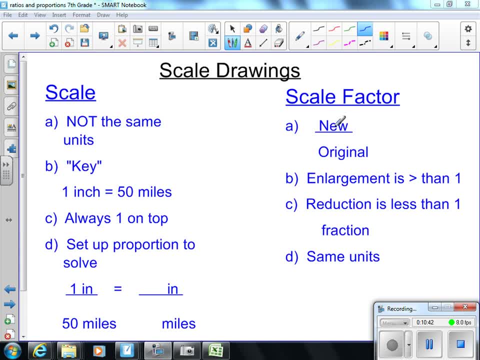 Now the scale factor. Now, the scale factor Is a fraction. It can be improper, But you always say the new over the original. In other words, if it's a reduction, Then my new is going to be smaller than my original. Therefore, it'll look like a fraction. 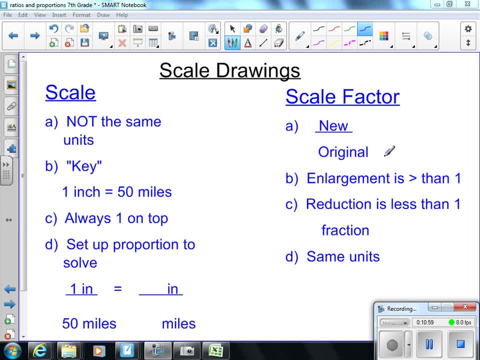 If it's an enlargement, Then my top number is going to be bigger than my bottom number And any number that does that is going to be greater than 1. Or, as I stated earlier, If it's a reduction, Then this is going to look like a fraction. 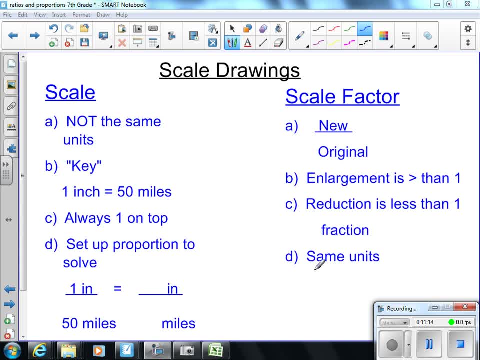 Or it's a number less than 1.. And this last note is really huge. You have to have the same units When you're figuring the scale factor. That's the key Right here. You'll have same units And for your purposes, 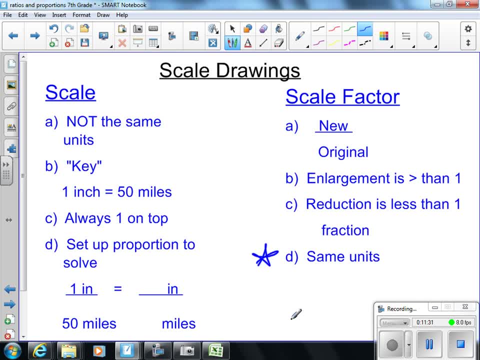 That's what you're going to do: Just convert them to make sure that they have the same units And simplify. So you may have to just do convert And then simplify, Okay, so let's take a look at an example Now. this is using your scale. 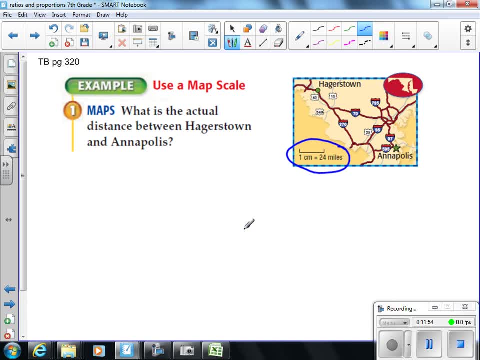 And how you use it. on maps. They give you a key at the bottom. Do you notice that? What is that key? 1 centimeter represents 24 miles. Okay, that's our first ratio that we know. They want to know the actual distance. 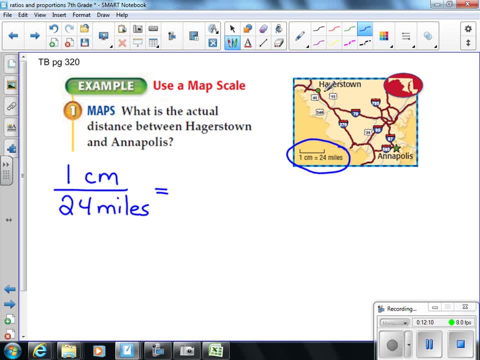 Between Hagerstown and Annapolis. So with your rulers right now And your book, I need you to measure in centimeters How far it is from Hagerstown to Annapolis. Go down there as half centimeter if you need to. 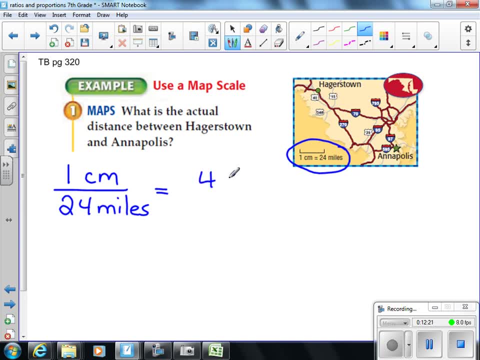 What did you get? 4? Okay, everybody is saying 4 centimeters, Thumbs up if you agree with that. Okay, do I know how many miles? Nope, So let's put X miles, Or you can put N, Any kind of variable. 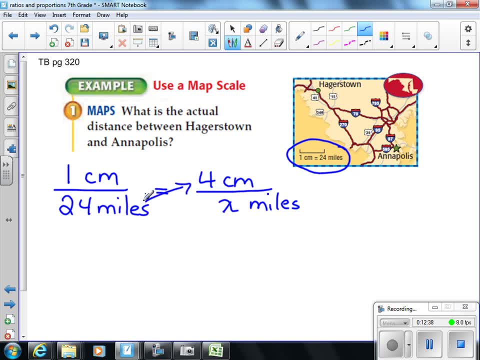 And what do I do to solve Cross products 24 times 4.. 96.. 96 equals 1X Divide by 1.. Remember we talked about showing your steps And you get 96 miles. So in real life it's going to be 96 miles from Hagerstown to Annapolis. 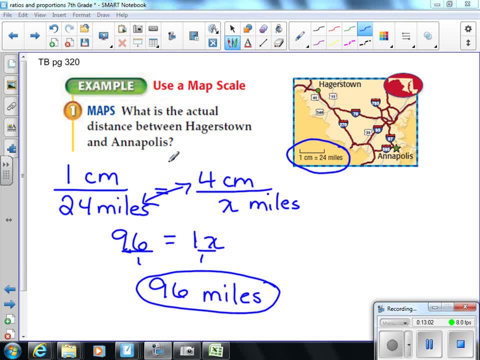 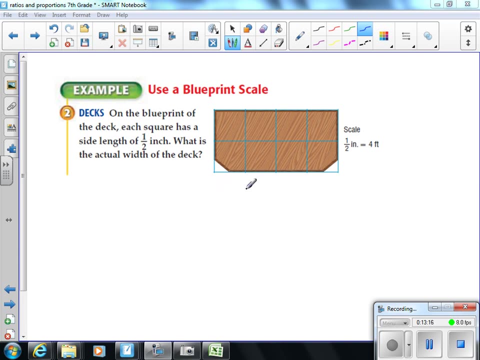 Approximately Okay. so basically, when you have your numbers, You have a scale on a map or a drawing. You're basically setting up a proportion and solving: Okay, this one is from a drawing. It says on the blueprint of the deck: Okay, this is a deck here. 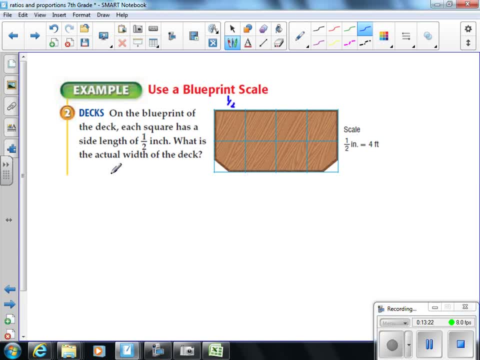 Each square has a side length of half an inch. Okay, so this represents a half an inch. What is the actual width of the deck? Well, here's the scale that they gave you, So let's write that down: One half of an inch compared to 4 feet. 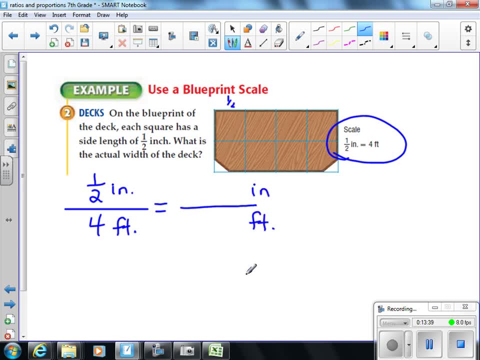 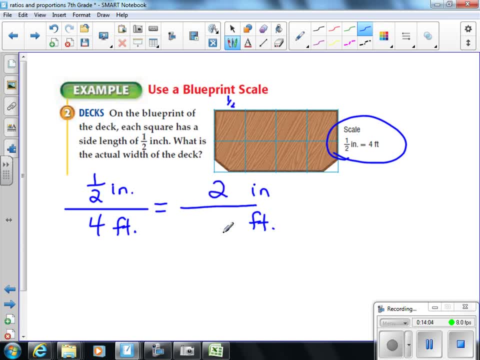 So a half inch represents 4 feet. This is 2 inches, Okay, and then this would be x feet. Now, what do I do? Cross products 4 times 2 is, And then I have one half times x. Ooh, what do I do now? 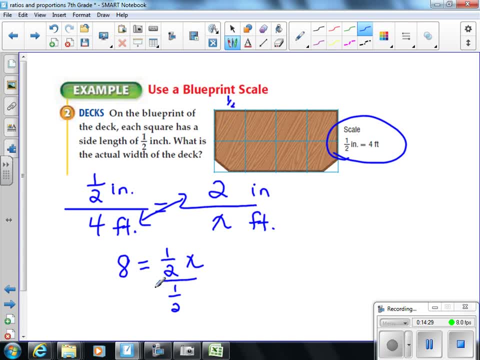 I am multiplying by a half, So I have to divide both sides by a half. Ooh, we have to review fractions. What do I do? 8 times 2 over 1. Multiply by its reciprocal, So go to KFC. 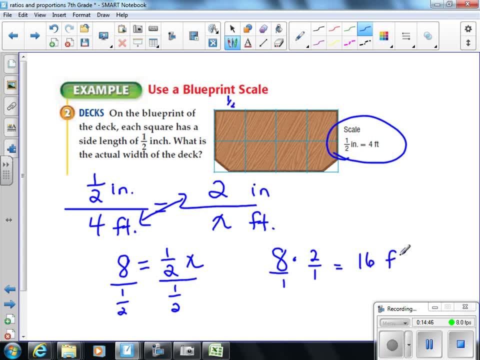 Flip it And you get 16.. So it would be actually 16 feet. Now let's see if that makes sense, Because it said each half inch here represents 4.. So that's 4, 4,, 4 feet, 4 feet. 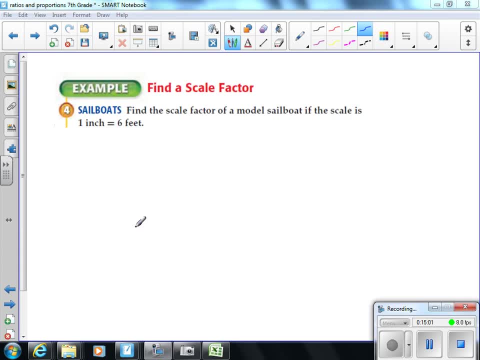 Is that right? Will it be 16?? Okay, great, Alright, let's take a look at a scale factor problem. It says find the scale factor And notice. it doesn't say just scale of a model sailboat if the scale is 1 inch to 6 feet. 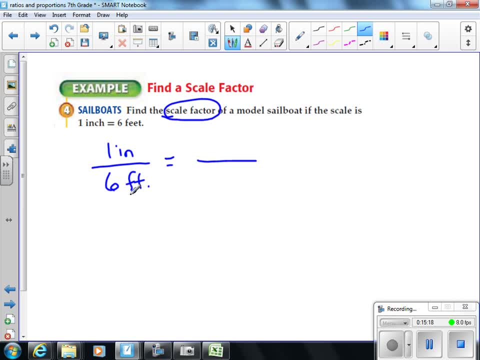 Now, if you look at your notes, what did we say had to happen? if you're finding the scale factor: Same units. So what do we have? to change feet to Inches? How do I do that? Right, 6 times 12 is. 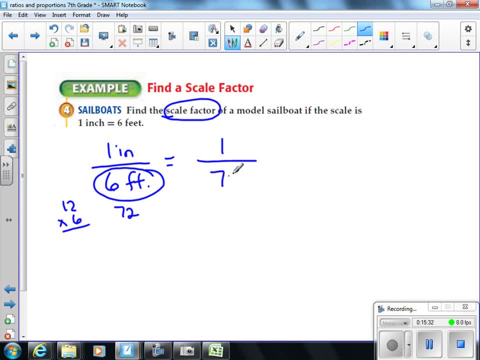 72.. Therefore, my scale factor is 1. To 72.. Now, this is not setting up cross products or setting them as a proportion. This is just like an equivalent ratio, Making it so that it's simplifying fractions. Just make, because the 1 is already at the top. 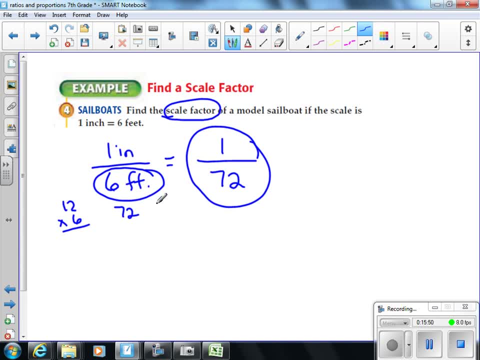 I'm done. When the scale factor you need to make sure your labels are the same- 1 inch to 72 inches- Or we kind of just throw your labels out. then They say the scale factor is 1 to 72.. 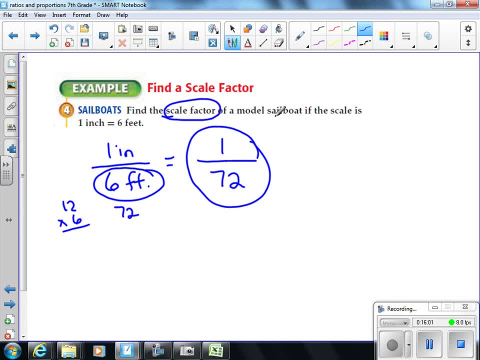 In other words, this is a reduction. I'm not going to put the real sailboat in there. In order to get my picture, I'm going to have to reduce it. Okay, that concludes our lesson on scale drawings and scale factors.